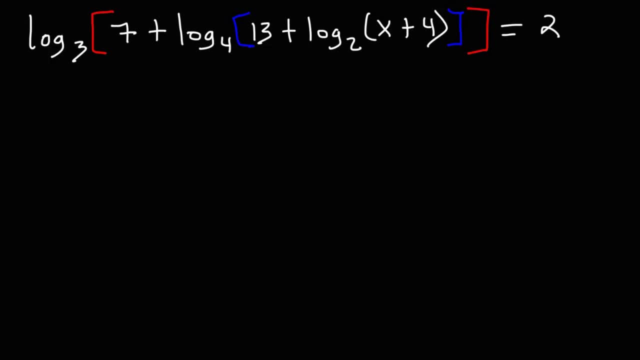 Consider this complex logarithmic equation. What would you do to solve it? Feel free to pause the video. if you want to give this problem a shot, Go ahead and try it Now. before we tackle this problem, there are some things we need to review. That is, the ability to convert a logarithmic 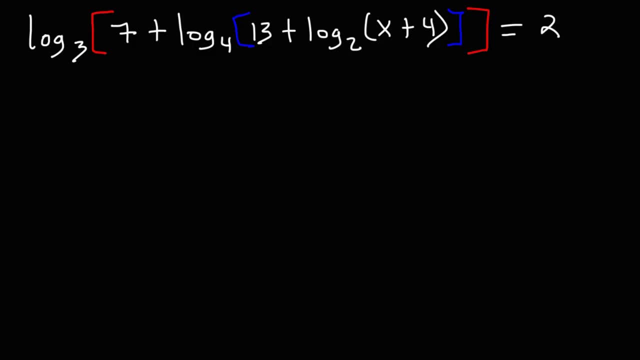 expression into an exponential one. For instance, consider this formula: log base A of B is equal to C. We can convert it into its exponential form by following this process: A raised to the C is equal to B. So let's say we have log base 4 of 64 is equal to 3.. We could say that: 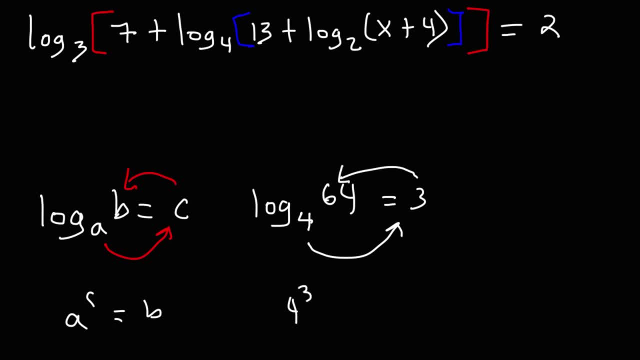 four raised to the third, power is equal to 64.. So we're going to do a lot of that in this particular problem. So let's begin. The first thing we could do is say: three raised to the second, power is equal to everything else here, everything in the red brackets. So let's write that: three squared. 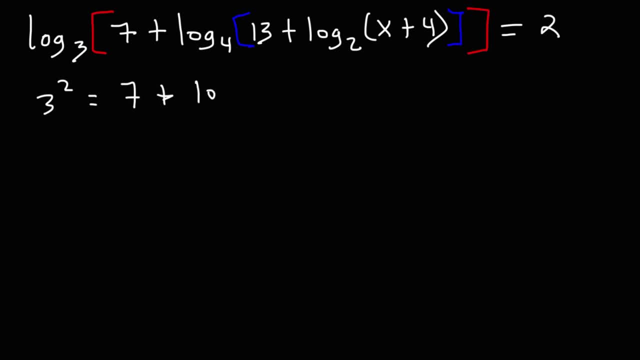 is equal to 7 plus log base 4 of 13 plus log base 2 of x plus 4.. Now, 3 squared is equal to 9, and so we have: 9 is equal to 7 plus everything else. So what is our next step here? Our next step is to subtract both sides by 7.. If we do that, 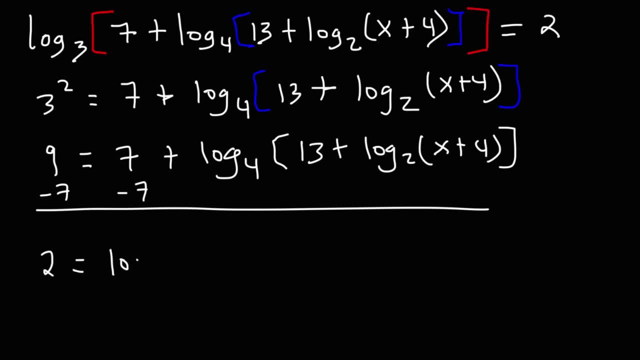 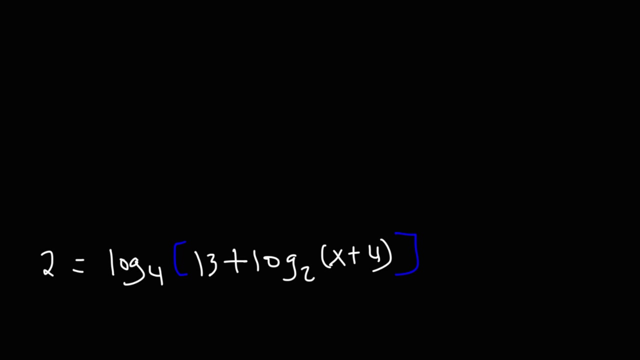 we're going to have. 2 is equal to log base 4 of 13 plus log base 2 of x plus 4.. Now notice that we can repeat the process. We now have another logarithmic expression and we can convert that into an exponential one. So we could say that 4 raised to the second power. 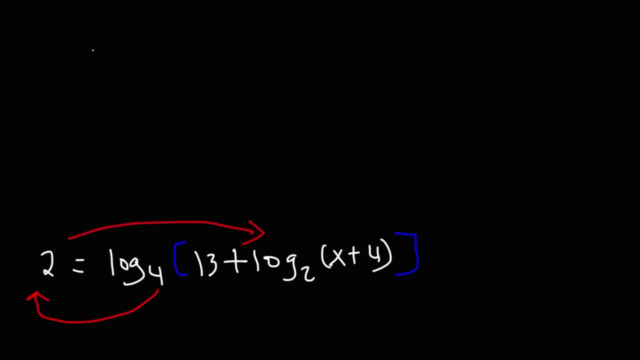 is equal to everything that we see inside. So 4 squared is equal to 13 plus log base 2 of x plus 4.. 4 squared is 4 times 4, and 4 times 4 is 16.. So now we need to subtract both sides by 13.. 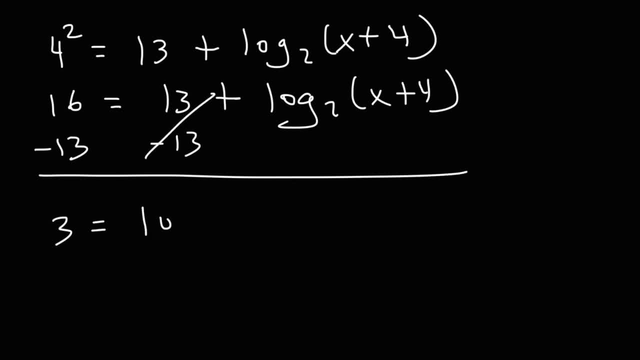 16 minus 13 is 3, so we're going to have: 3 is equal to log base 2 of x plus 4.. Now let's transform this one into its exponential form as well: 2 raised to the third power is equal to x plus 4.. 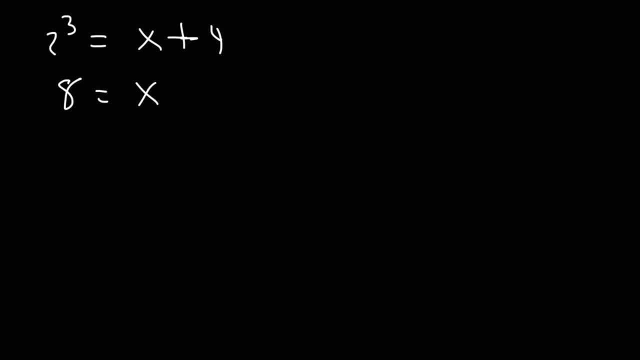 2 to the third, power is 8, and so we have: 8 is equal to x plus 4.. So we're going to subtract both sides by 4, and we're going to have: 8 minus 4 is 4, and that is equal to x. 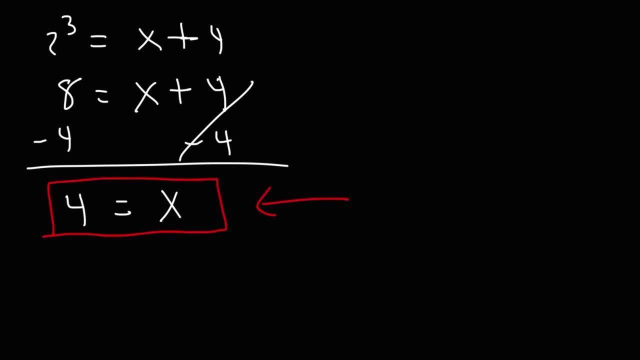 So this is the answer to the logarithmic problem. x is equal to 4.. As you can see, it's really not that bad. As long as you understand the properties of logarithms, you can solve it. Now let's make sure that the answer that we have is indeed correct. 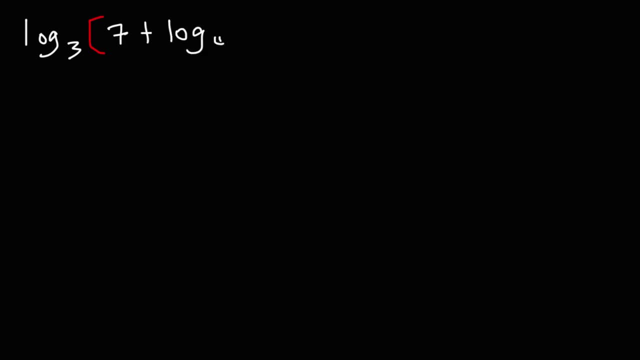 So what I'm going to do right now is I'm going to rewrite the problem. So I'm going to rewrite the problem and then replace x with 4 to see if the answer is indeed correct. So this is the original problem. If we replace x with 4, we're going to have 4 plus 4, which is 8.. 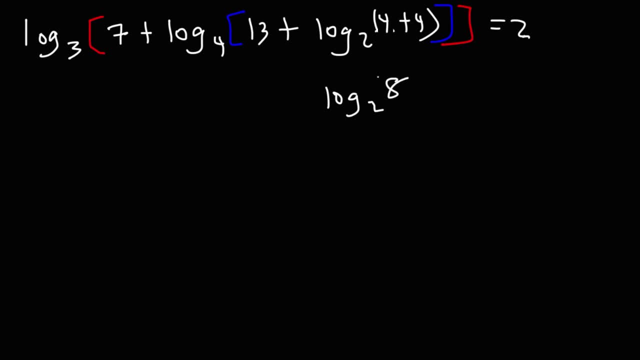 So we have log base 2.. So we have log base 2 of 8, and then plus 13.. So what is log base 2 of 8?? 2 raised to the, what power is equal to 8?? We know, 2 to the third power is 8.. 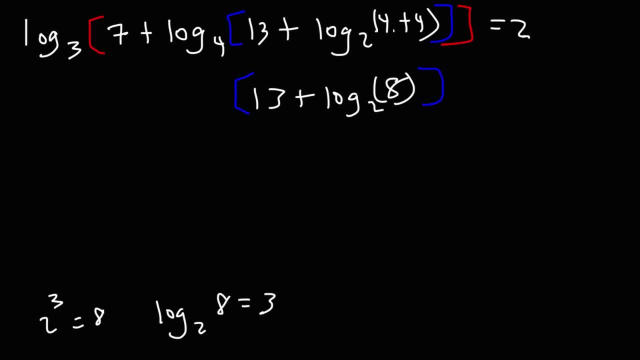 So log base 2 of 8 is equal to 3.. As you can see, 2 to the third is 8.. So we can replace log base 2 of 8 with 3.. And so right now we have 13 plus 3, which is 16.. 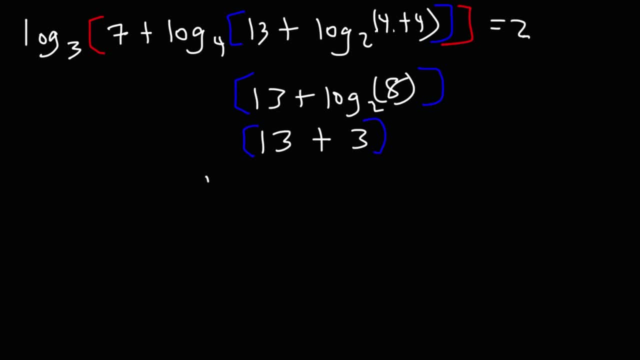 So we have log base 4 of 16, and then we have a plus 7 outside of that. Now, what is log base 4 of 16?? 4 raised to the, what power is equal to 16?? Well, we know that 4 squared is 16.. 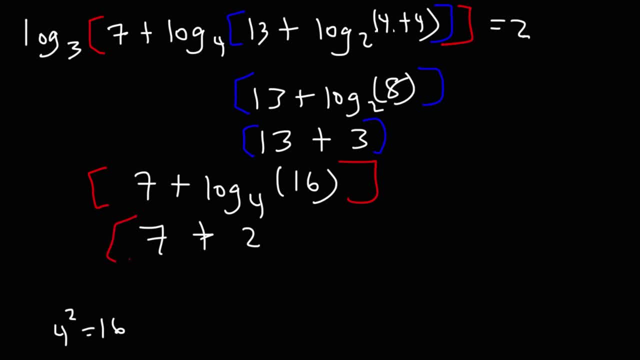 So log base 4 of 16 is 2.. And then we have 7 plus 2,, which is 9.. And then we're left with log base 3 of 9.. 9 is equal to 2. And we can clearly see that 3 squared is 9.. 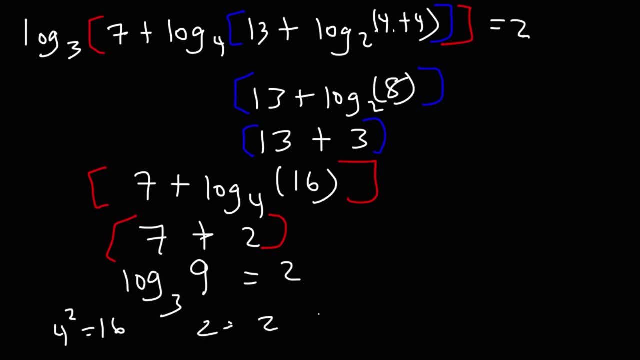 So log base 3 of 2 is 2,, which means the answer is correct. So that's a quick and simple way of how you can check to see if we indeed have the right answer. Now let's work on one more example problem. 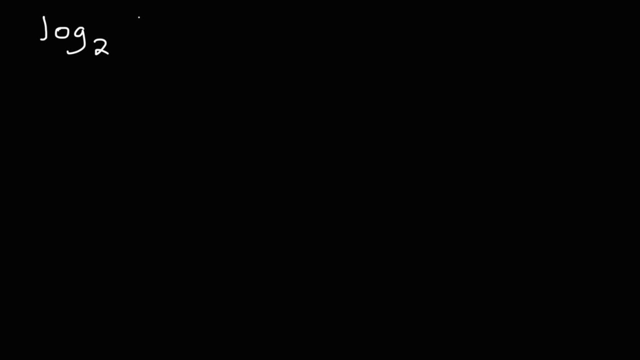 Let's say we have log base 2 of log base 4 of x, x raised to the 16th power, And let's say all of that is equal to 3. Go ahead and try this problem. So what do you think is the first thing that we need to do here? 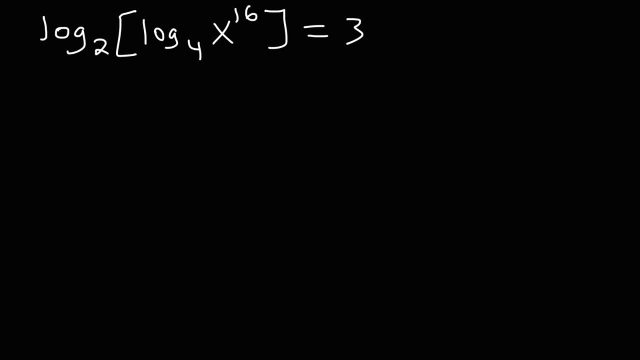 Based on what we've done before, we need to convert the logarithmic expression into an exponential one. Starting with base 2, we could say that 2 raised to the 3rd power is equal to everything inside of the brackets. So 2 to the 3rd is equal to log base 4 of x raised to the 16th. 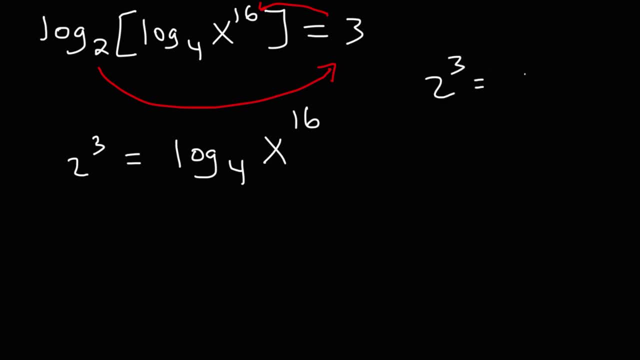 Now 2 to the 3rd power. we're multiplying 3 2's together, So this is equal to 8.. So we could say that 8 is equal to log base 4 of x raised to the 16th. 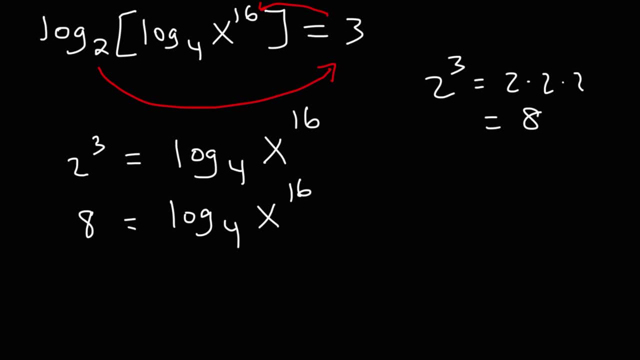 Now we could repeat the process. What we could do is we can say: 4 raised to the 8th, power is equal to x to the 16th. That's one option, But let's write that over here. Another thing we could do is we could move this 16 to the front. 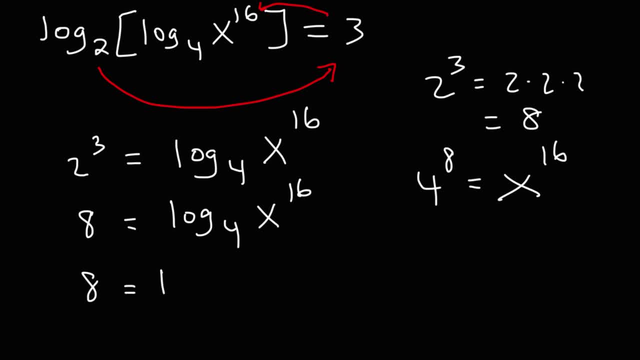 That's another property of logs. So we could say that 8 is equal to 16 times log base 4 of x. Personally, I think this is just easier to deal with. I mean, both methods will work. It will get you the right answer, but this looks a lot simpler. 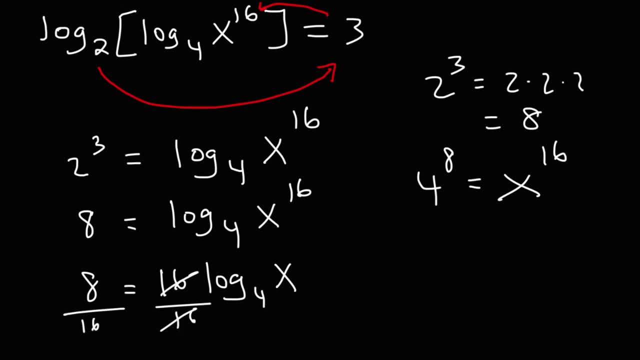 Let's divide both sides by 16.. 8 divided by 16, we could reduce that to 1 half. If you want to show your work, here's what you can do: Replace 16 with 8 times 2. And 8, replace it with 8 times 1.. 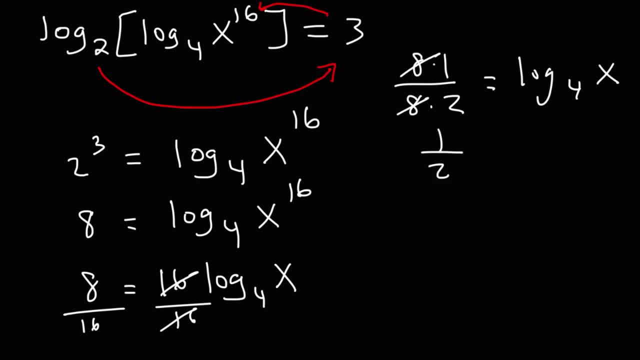 And so canceling the 8. You're left with 1 half. So we have: 1 half is equal to log base 4 of x. 4 raised to the 1 half is equal to x. Now, whenever you raise something to the 1 half, you're basically taking the square root of that number. 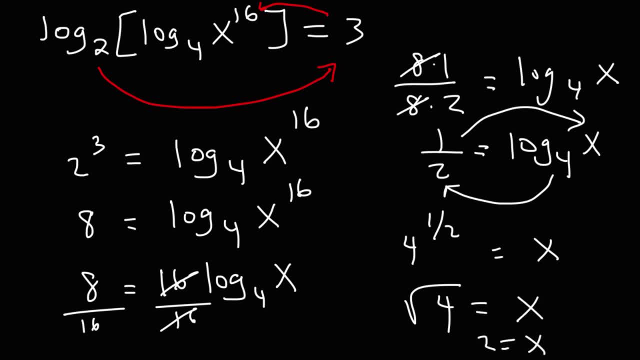 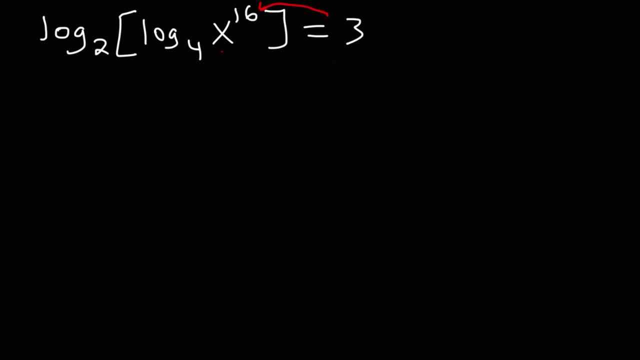 And the square root of 4 is 2.. So therefore, x is equal to 2.. Now, just to make sure that we indeed have the right answer, let's go ahead and plug this in to our original equation. So we have log base 2 of log base 4.. 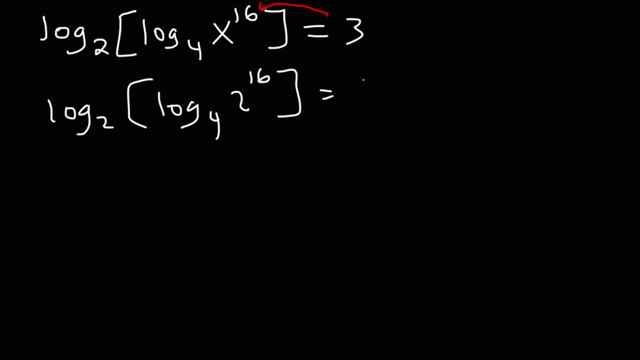 And then 2 raised to the 16.. Now it would definitely be good to move the 16 to the front. So we have 16 log base 4 of 2.. Now I'm going to use the change of base formula to evaluate log base 4 of 2.. 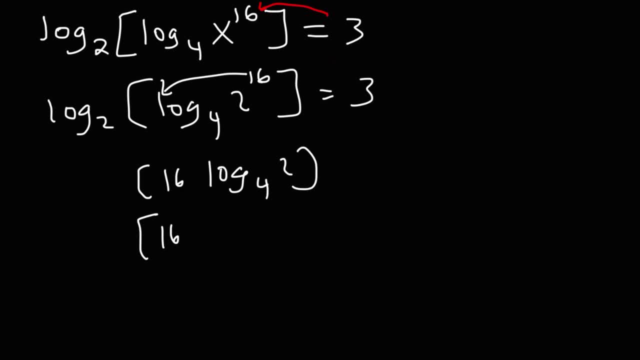 You could say that the answer is 1 half, because 4 to the 1 half is equal to 2.. I'm going to do it a different way. So log base 4 of 2 is equal to log 2 over log 4..